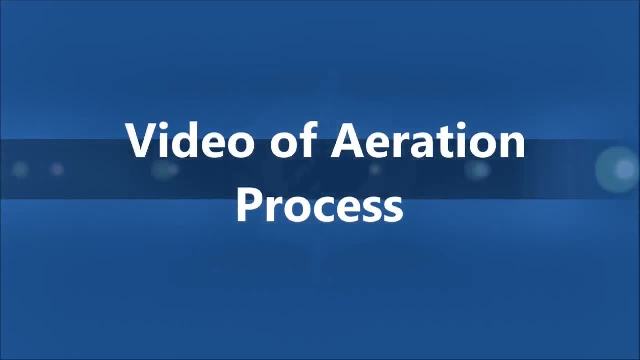 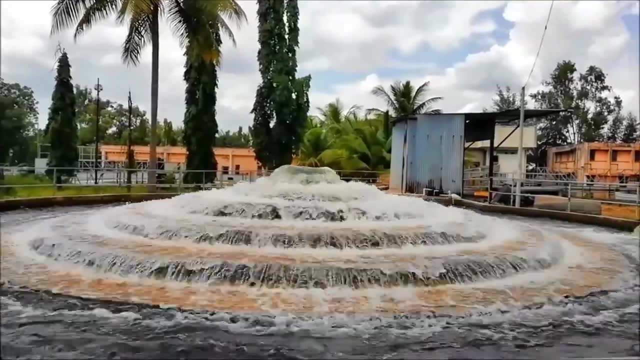 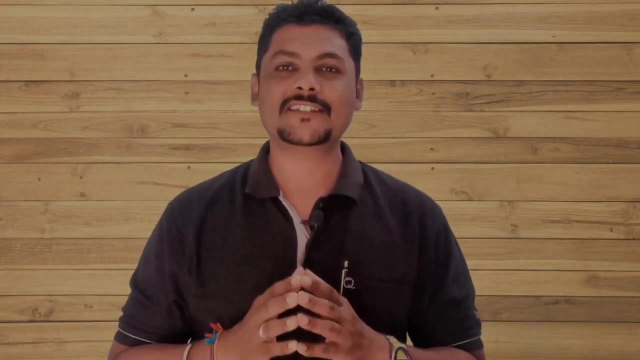 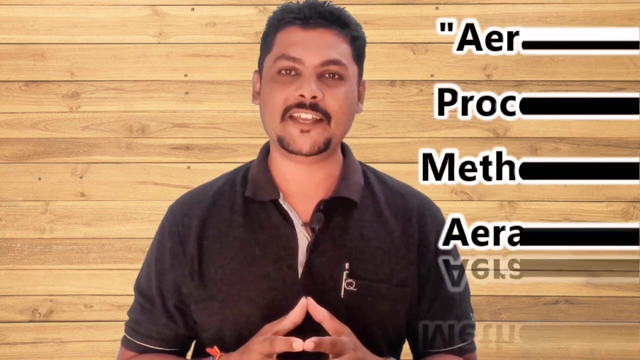 Before starting the lecture, let's see a short clip of aeration process. Hello, my dear viewers, Welcome to simplified civil and geotechnical engineering channel. I am Akshay Jaiswal. In this video, I am going to explain aeration process and methods of aeration. So let's start today's lecture. 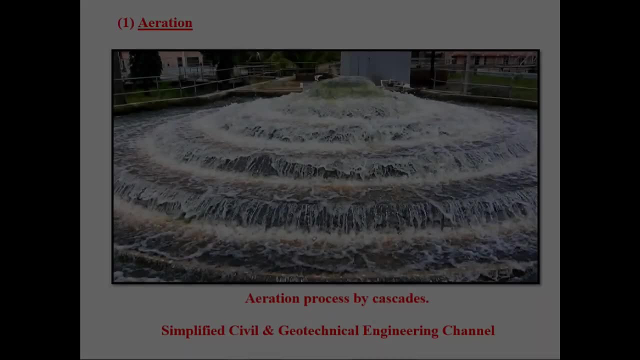 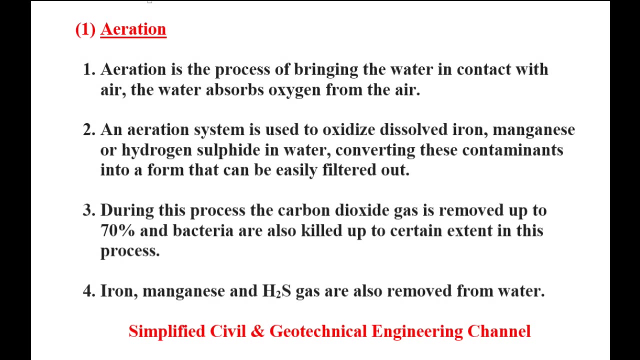 Chapter number 2. Purification process- Purification of water. This picture shows aeration process by cascades. Now we will discuss about aeration process, Point number 1.. Aeration is the process of bringing the water in contact with air, and water absorbs oxygen from the air. 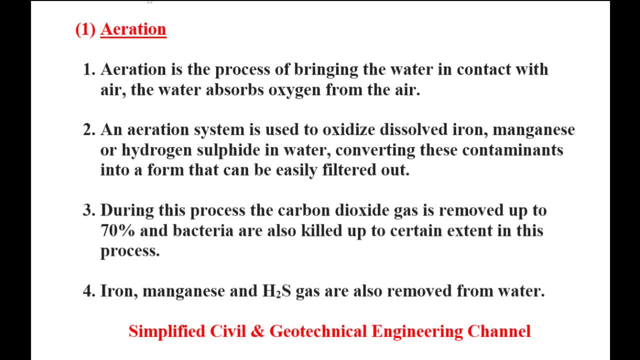 Point number 2.. An aeration system is used to oxidize dissolved iron, manganese or hydrogen sulfide in water, Converting this content into a solution Contaminants into a form that can be easily filtered out. Point number 3.. During this process, the carbon dioxide gas is removed up to 70% and bacteria are also killed up to a certain extent in this process. 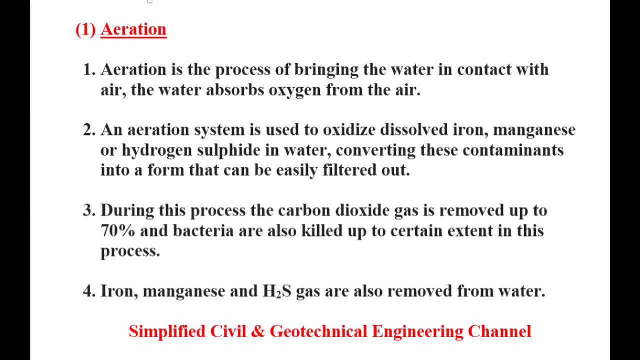 Point number 4.. Iron, manganese and H2S means hydrogen sulfide gas- are also removed from water. So let's see the aeration process in detail. Aeration means water. In the process, the carbon dioxide gas is removed up to 70%. 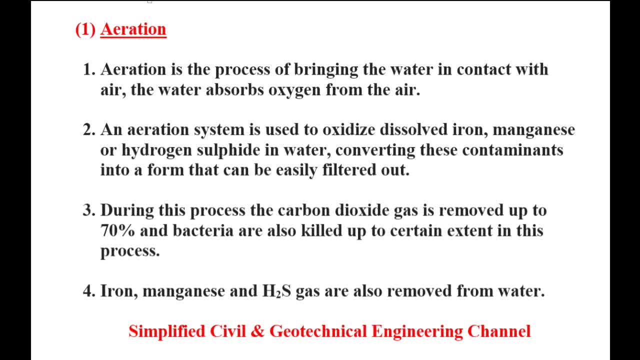 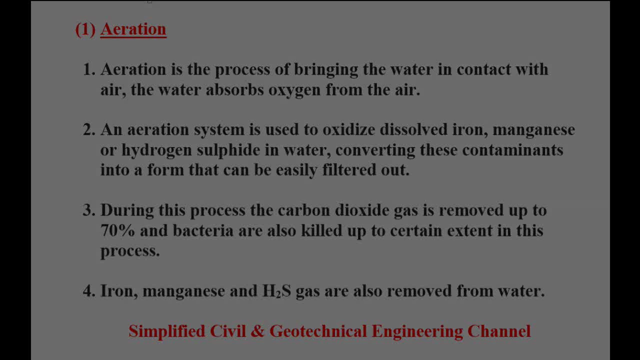 Along with this, the bacteria are also removed up to a certain extent. Iron, manganese and H2S means hydrogen sulfide gas is also removed from water. Objectives of aeration Point number 1. Removal of hydrogen sulfide from raw water and the removal of hydrogen sulfide from raw water. 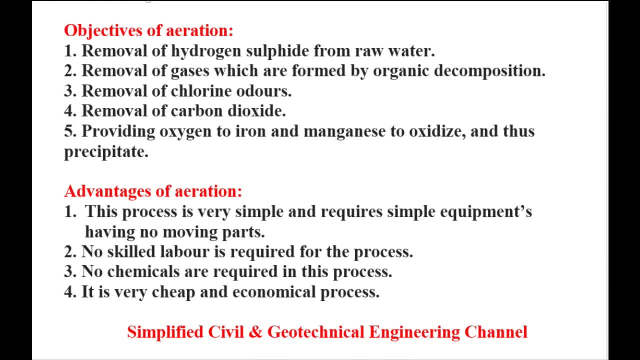 In this process, water is absorbed by oxygen from raw water. point number two: removal of gases which are formed by organic decomposition. point number three: removal of chlorine orders. point number four: removal of carbon dioxide. point number five: providing oxygen to iron and manganese to oxidize and thus precipitate. 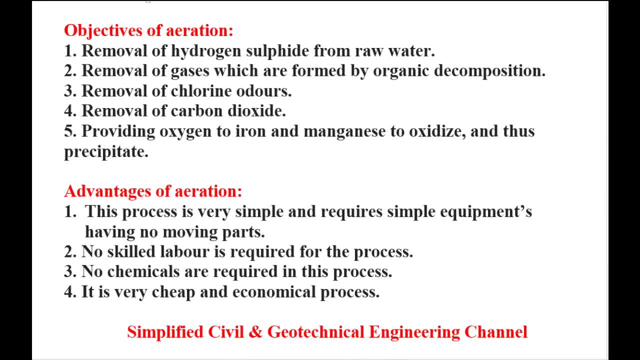 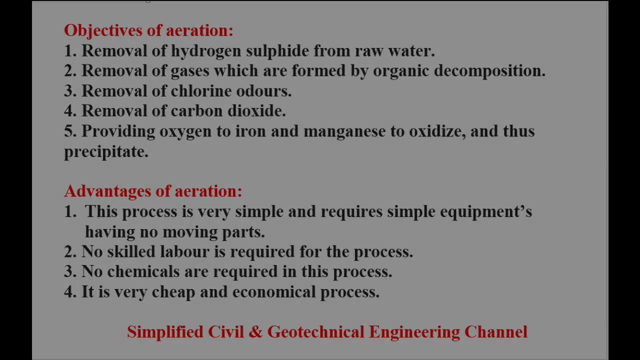 advantages of aeration. point number one: this process is very simple and requires simple equipments having no moving parts. point number two: no skilled labor is required for the process. point number three: no chemicals are required in this process. point number four: it is very cheap and economical process. this picture shows aeration process by cascades. 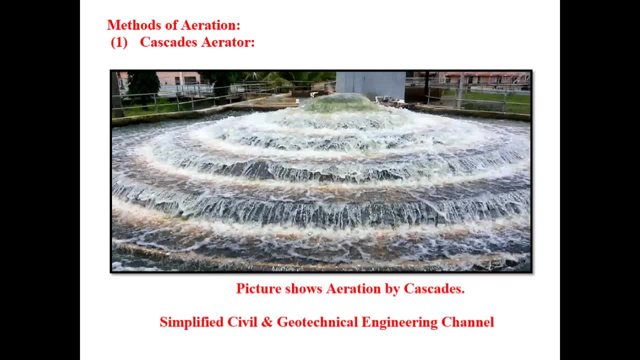 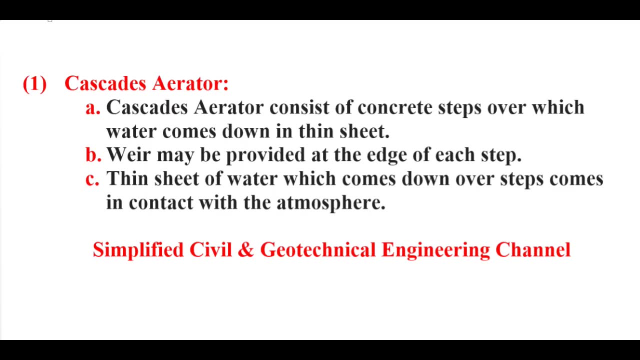 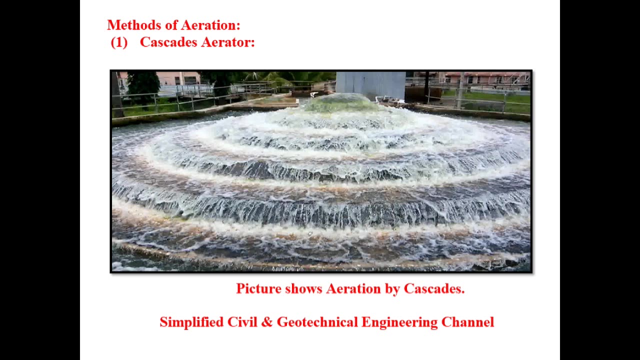 Now we will discuss about cascade aerator. cascade aerator consists of concrete steps over which water comes down in thin sheets. Point number B: wear may be provided at the edge of each step. Point number C: thin sheet of water which comes down over steps comes in contact with. 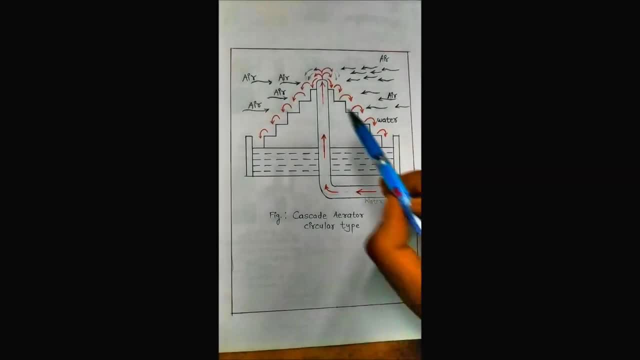 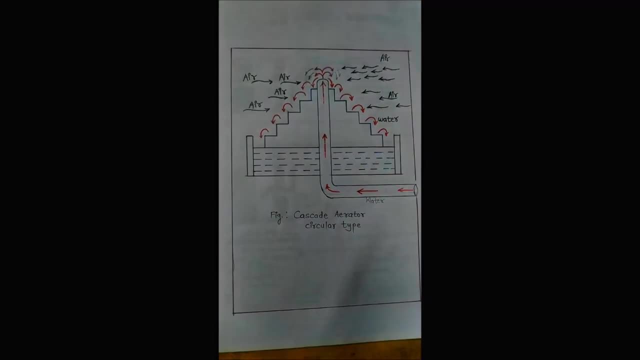 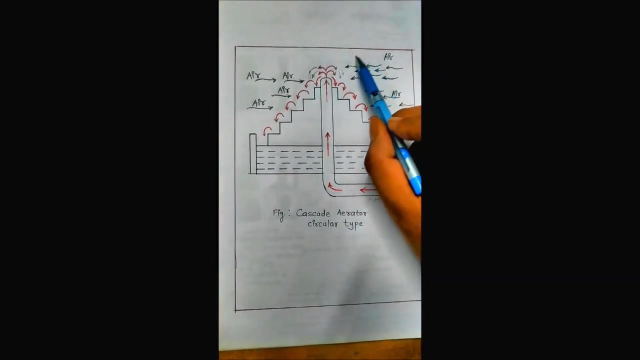 the atmosphere Aeration process. it consists of concrete steps over which water flows down in the form of thin sheets. When water goes down over the steps, it comes in contact with atmospheric air. More surface of water is exposed to the surrounding air, which removes gases from the water. 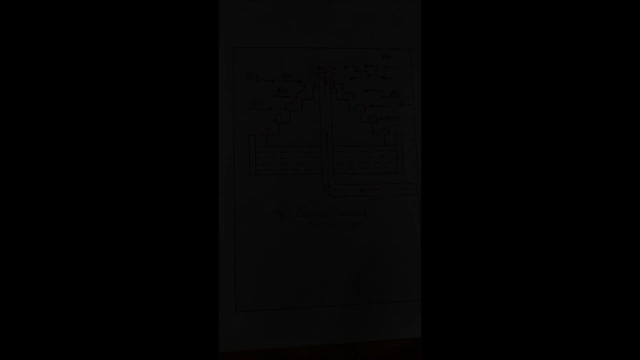 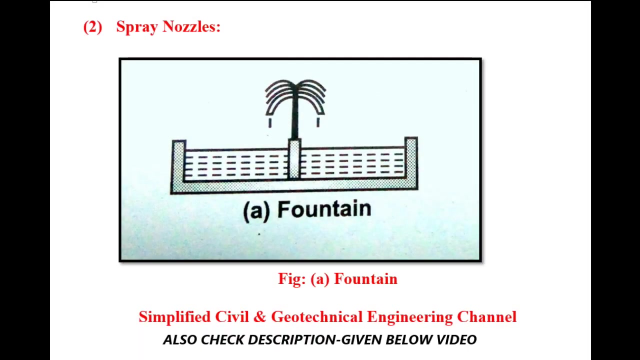 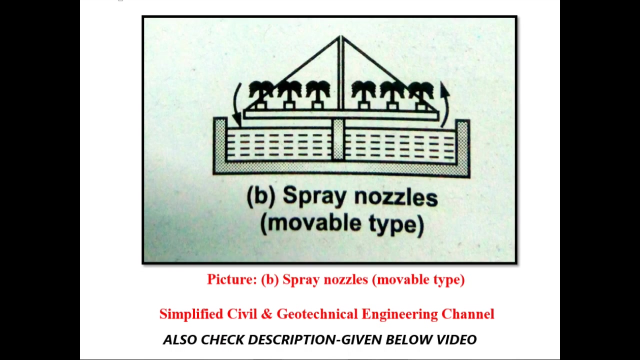 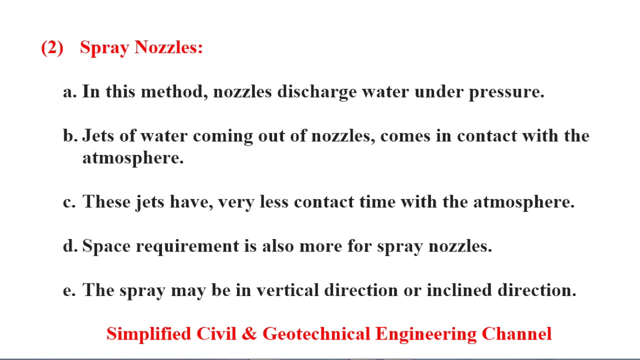 Due to aeration, more oxygen is absorbed by water. This picture shows A huge mountain in which we can see jets of water coming out of nozzles. Picture B shows spray nozzles which have moving part and nozzles. Picture C shows spray nozzle having fixed pipe. 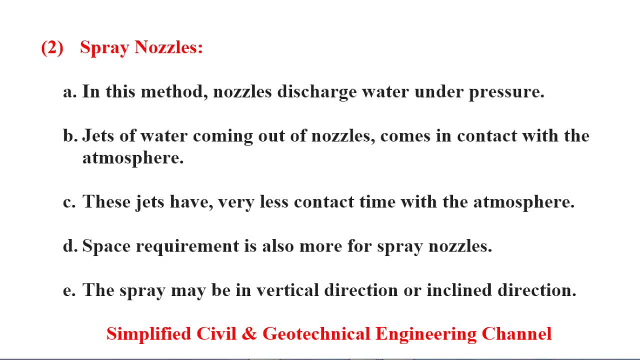 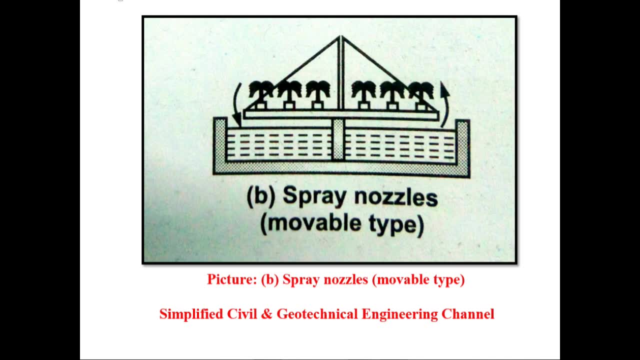 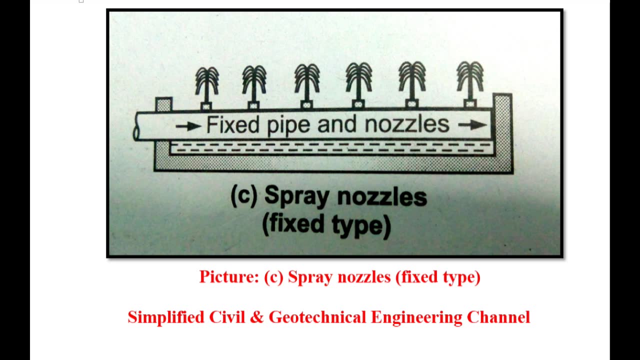 Now lets see spray nozzles, Point number A in this method. nozzles discharge water under pressure Jets of water coming out of nozzles comes in contact with atmosphere. These jets have very less contact time with atmosphere. requirement is also more for spray nozzles. the spray may be in vertical. 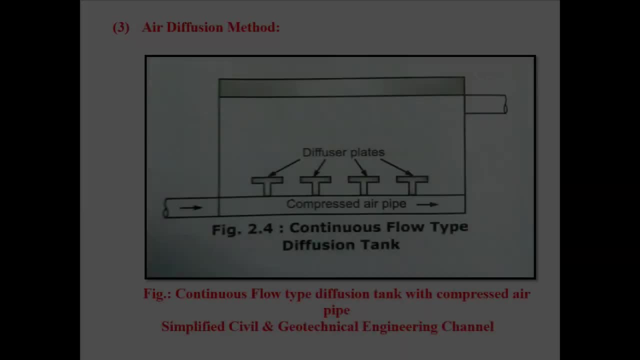 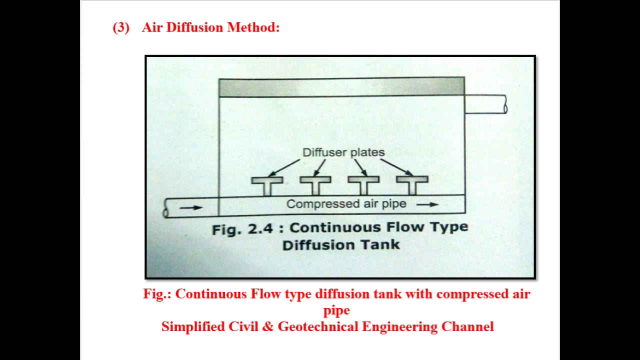 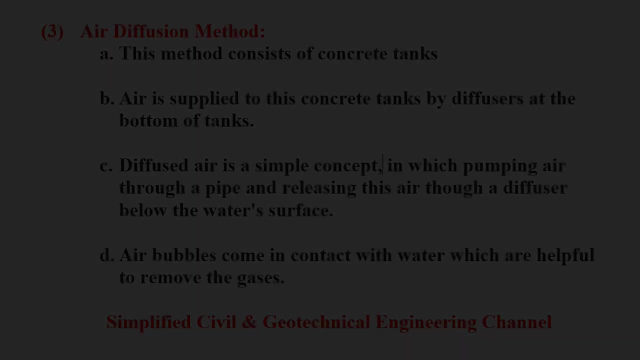 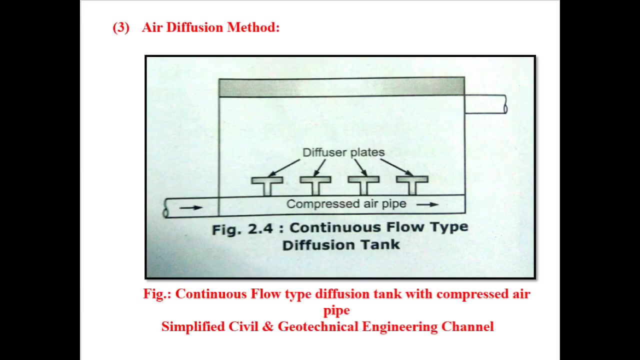 direction or inclined direction. this figure shows compressed air pipe. in this method, compressed air is supplied through the diffuser plates. air bubbles comes out from this plate, which are useful to remove dissolved gases from water. now let's discuss about air diffusion method. point number a: this method consists of concrete tanks. point number B: air is supplied to this. 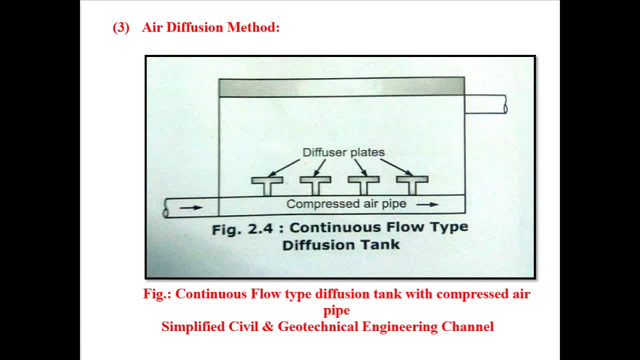 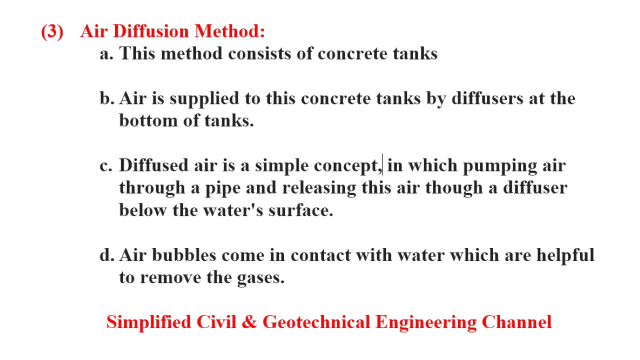 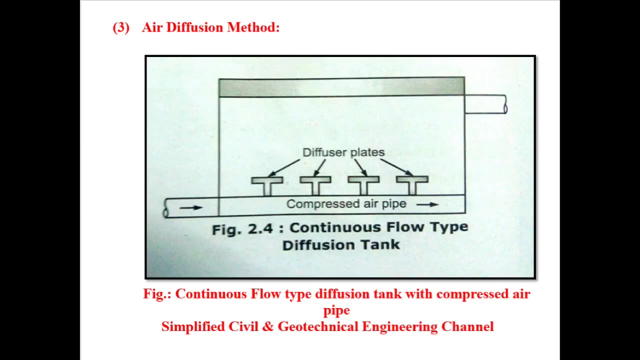 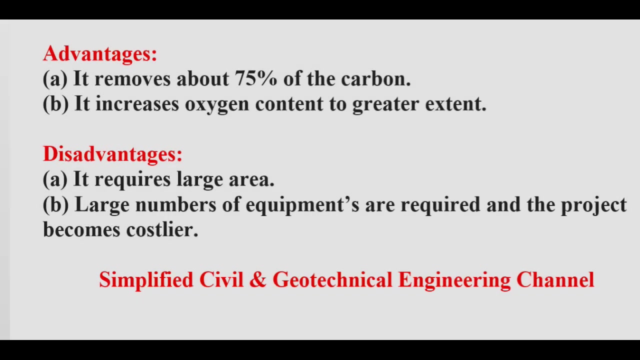 concrete tanks by diffusers at the bottom of tank. point number C: diffused air is a simple concept in which pumping air through a pipe and releasing this air through a diffuser below the water surface- point number D- air bubbles- comes in contact with water, which are helpful to remove the gases. now let's see. 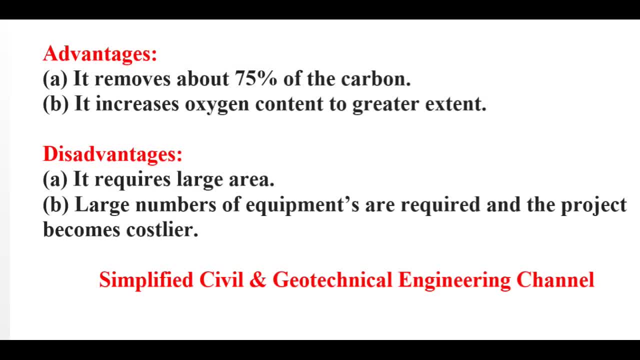 advantages and disadvantages of this method. advantages and disadvantages of air diffusion method. advantages are: it removes about 75 percent of carbon and it increases oxygen content to greater extent. now, disadvantages: it requires large area and large number of equipments are required and the project become costlier. this figure shows. 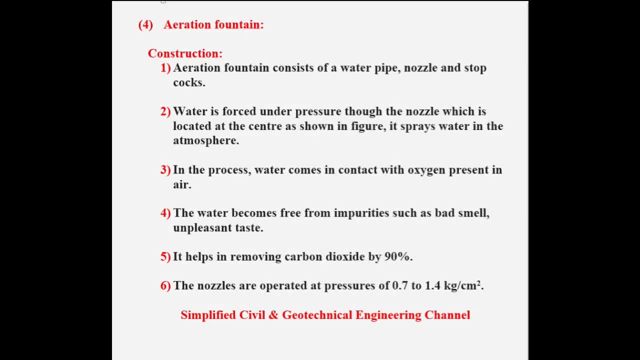 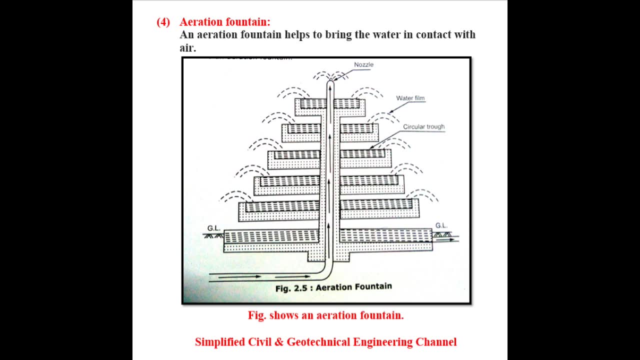 and aeration fountain. now we will discuss aeration fountain. let's start with its construction. point number one: aeration fountain consists of water pipe, nozzle and stopcocks. point number two: water is forced under pressure through the nozzle, which is located at the center. as shown in figure, it sprays. 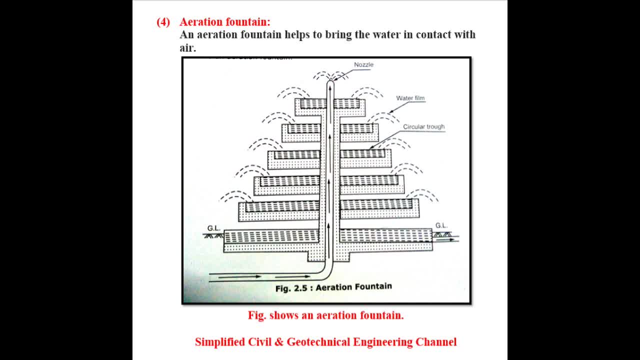 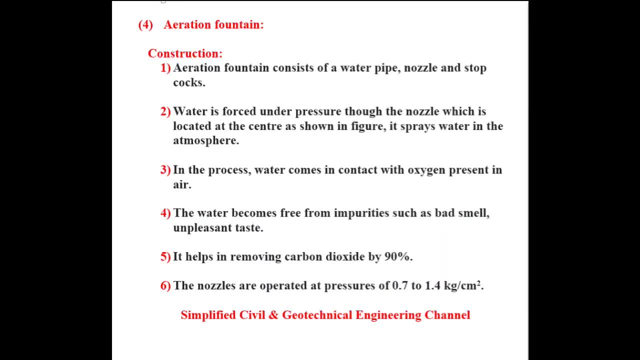 water in the atmosphere. point number three: in the process, water comes in contact with oxygen present in air. point number four: the water becomes free from impurities such as bad smell and unpleasant taste. point number five: it helps in removing carbon dioxide by 90%. point number six: the nozzles are. 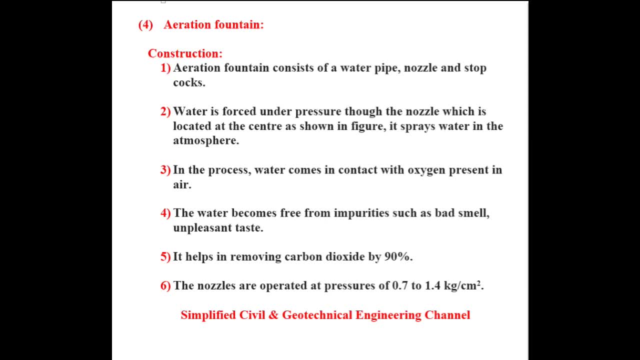 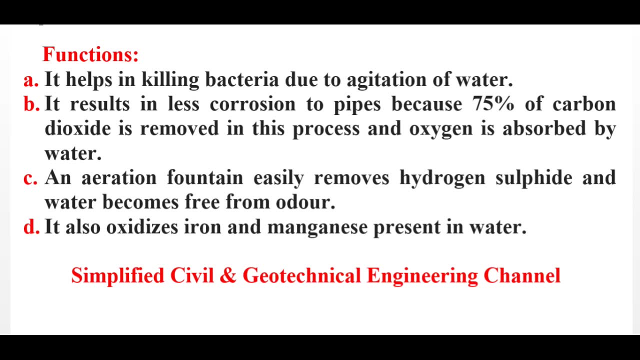 operated at pressure of 0.7 to 1.4 kg per centimeter square. now let's discuss functions of aeration fountain. point number four: the nozzle is free from impurities such as bad smell and unpleasant taste. point number five: it helps in killing bacteria due to agitation of water. point number B: it 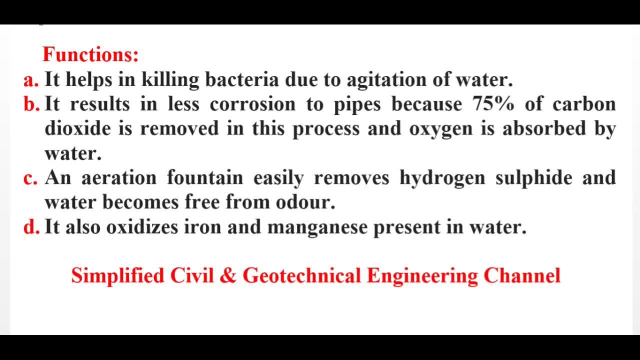 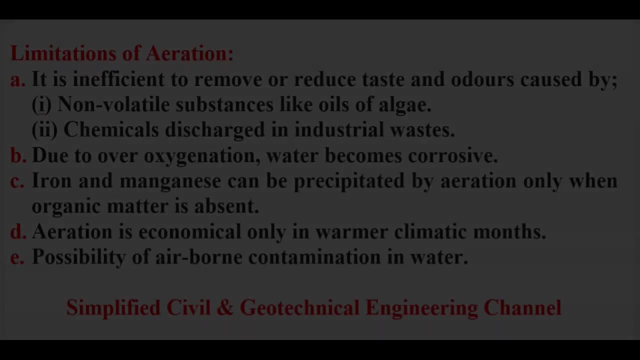 results in less corrosion to pipes because 75% of carbon dioxide is removed in this process and oxygen is absorbed by water. point number C: an aeration fountain easily removes hydrogen sulfide and water becomes free from odor. point number D: it also oxidizes iron and man is present in water.